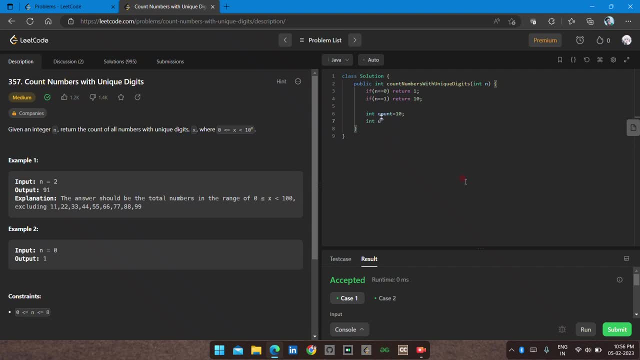 Other is unique numbers, which is: firstly, I will initialize it to 9.. Then I will level integers. I will initialize it to 9.. Then I will start the loop with integer i equal to 1, which will be i less than math dot minimum. minimum of what? 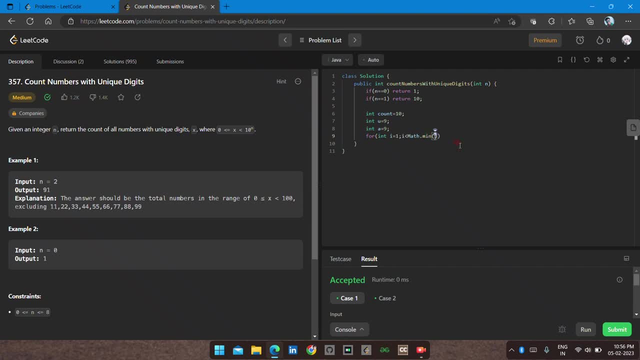 Minimum of what. Why n, comma 8.. Because if n is greater than 8, it will only loop continues till 8.. So I will. I am taking it as a reference And n is not greater than 8, as problem says it. 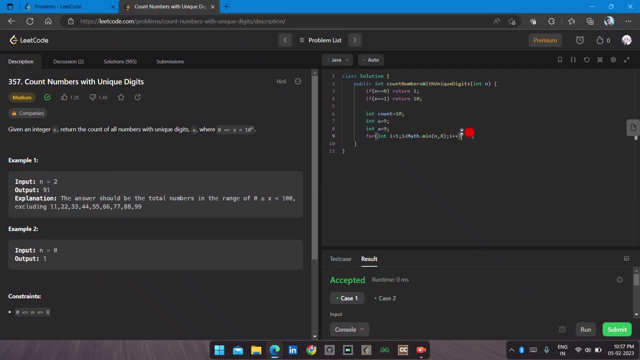 So let's consider here- And after that I will make here as what is unique integer here u is equal to into a Available number. Available number into unique integer is the unique integer. And then and then what? 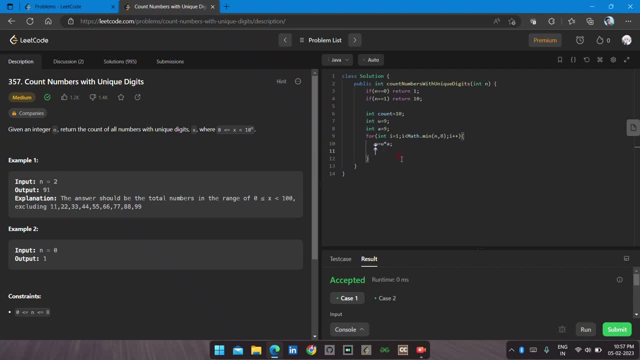 I will take it as available name. count plus is equal to. I will add this: I will add the unique integer into count and then I will minus the available integer by like this and I will return count and in this for loop, I think it is- I will place here as n, not other, because it is that thing n. 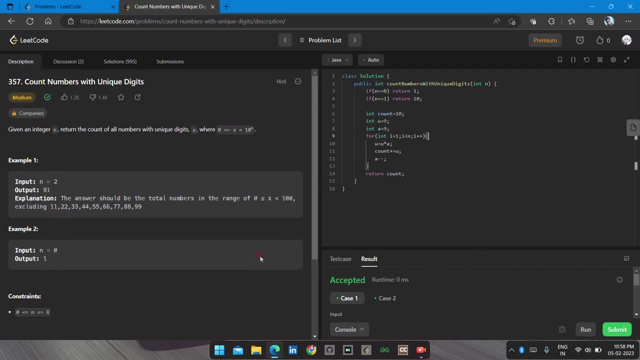 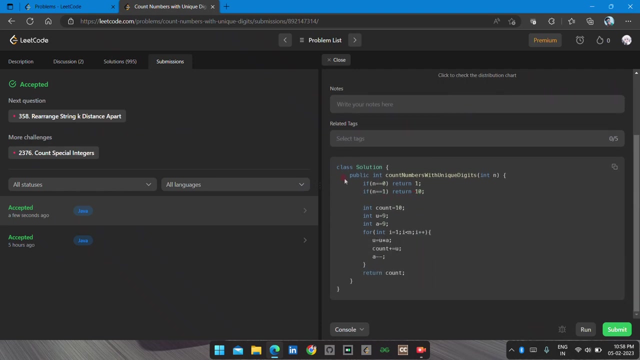 is not greater than 8, not greater than 8, so I will just submit it and let's take our answer, as I know it is right, so it beats 100%. I solved it using the dynamic programming approach. it is its time, complexity is O and space complexity is O as it uses the constant.